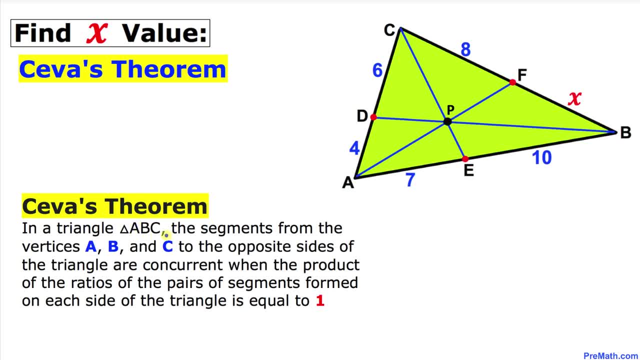 And here's our Siva's theorem. In a triangle ABC, the line segment P is 10.. The segments from the vertices A, B and C to the opposite sides of the triangle are concurrent. That means they pass through the very same point. in our cases P, when the product of the ratios of the pair of segments formed on each side of the triangle is equal to 1.. 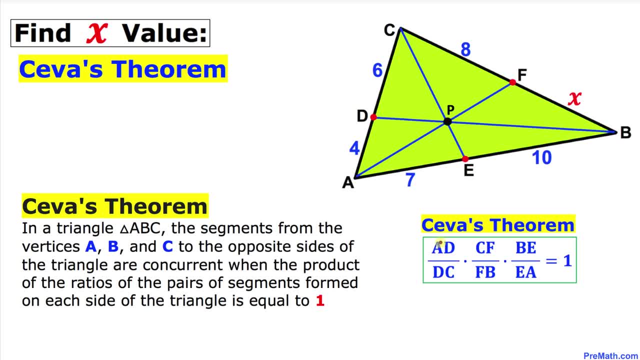 And here's our Siva's theorem: formula A- D. These are the ratios. By the way we are multiplying, the product of these ratios must be equal to 1.. And let me go over this thing: A D over D? C. As you can see, this is our A? D and this is D? C. The next ratio is C? F divided by F? B. 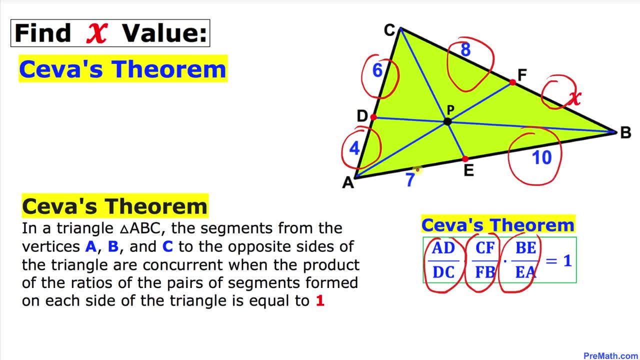 And the next ratio is B- E divided by E- A, That must be equal to 1.. And we got these ratios by going clockwise, isn't it? However, should you decide to go counterclockwise, so then our formula is going to be: simply becomes this one: 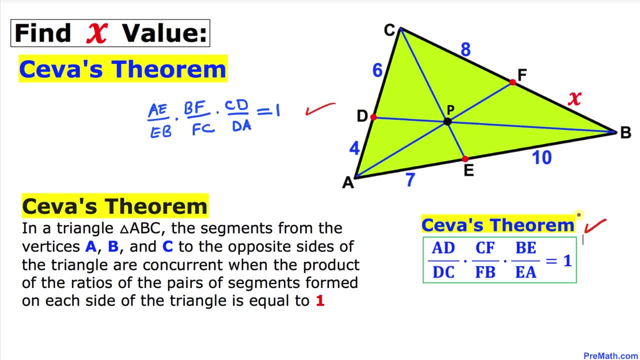 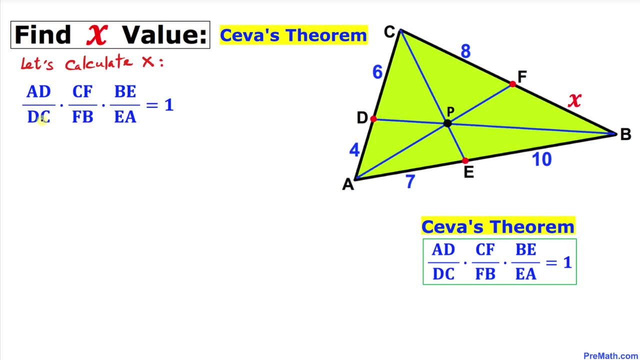 And both of these formulas are valid. Now let's go ahead and calculate the value of X, And here's our Siva's theorem. Let's go ahead and fill in the blanks: A, D, D, in our case, is simply 4.. 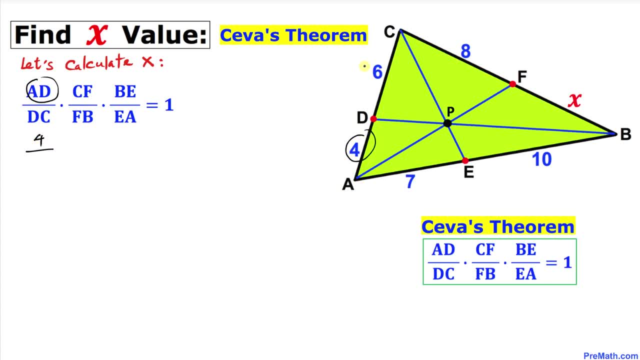 So I can write 4 over D: C, in our case, is 6.. And then times C- F, in our case, is 8.. So 8 divided by F, B, is this unknown- X, And then times B, E is 10 and A, A is 7.. 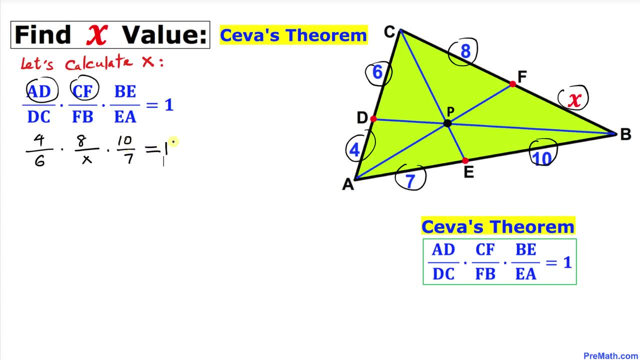 So it's 1 over D, C is 7.. And then times B, E is 10 and A, A is 7.. So let's go ahead and multiply the numerators and at the same time multiply the denominators On the top. we're going to get 320 divided by 42X, equal to 1..